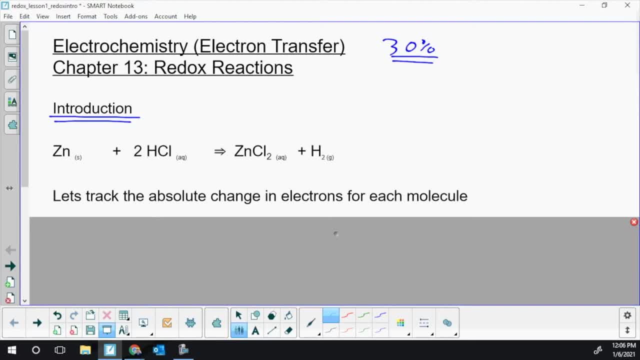 the reaction types from way back in Science 10.. This is a single replacement, And a single replacement reaction is an example of electron transfer reaction- We just never talked about it in Science 10, being a electron transfer one. To study whether something has electron transfer and is electrochemistry, we need to track electrons. So that's the 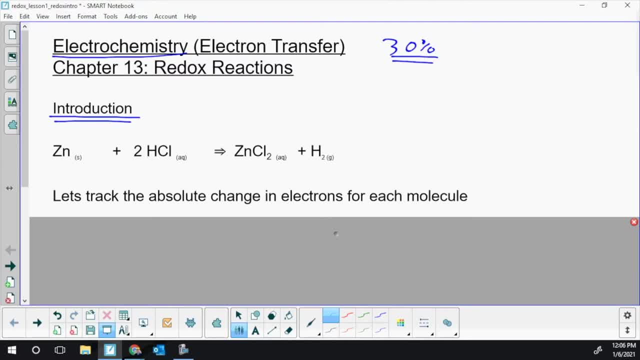 first thing I'm going to do, I'm going to look up how many electrons each species has. Okay, now to do that, I'm flipping to the data booklet and looking up that atomic cell symbol. So the very first thing we have is zinc, Zinc solid. You don't have to write. 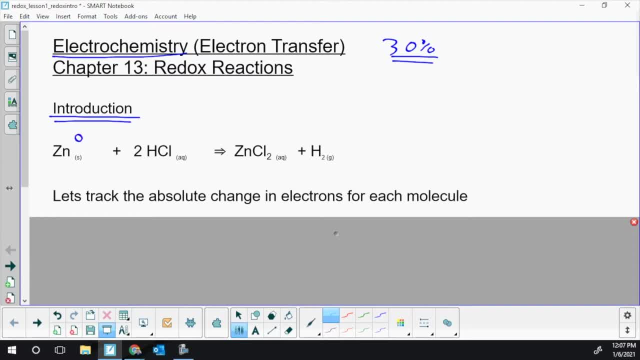 this in. but you have to realize that is neutral, has no charge. And if I look up zinc in your data booklet, zinc has 30 electrons. Okay, now what I'm going to do is put the total electrons on the bottom and on the top I'm just going to write the charge And in future, 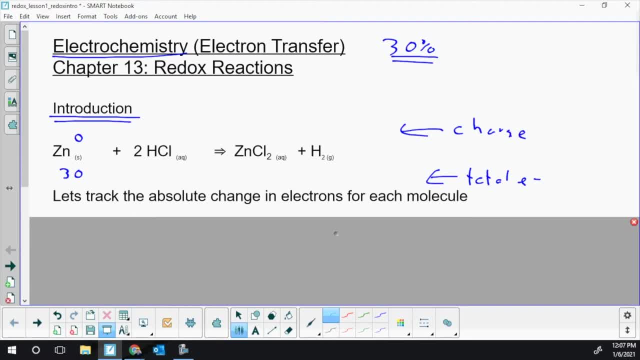 examples. I'm just going to do one of these two methods, but I want to give you the visual of the total electrons and how charge is a shortcut. okay, so zinc has 30 electrons. has no charge. if we look at HCl, okay, that HCl is a is a. 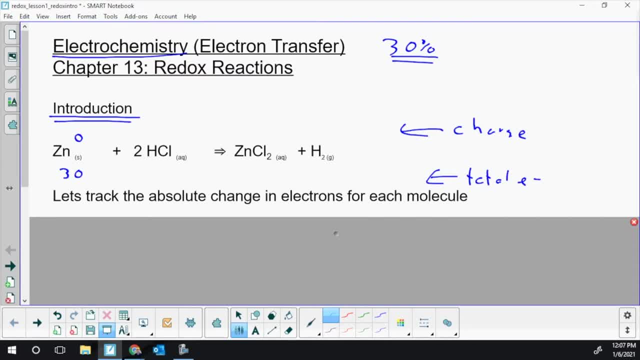 compound that is pretty close to being ionic, and I'm going to treat it ionic as that, H being a one plus and and a chloride one minus. if you think of H plus, well, hydrogen by itself would have one electron, but as H plus it has zero. 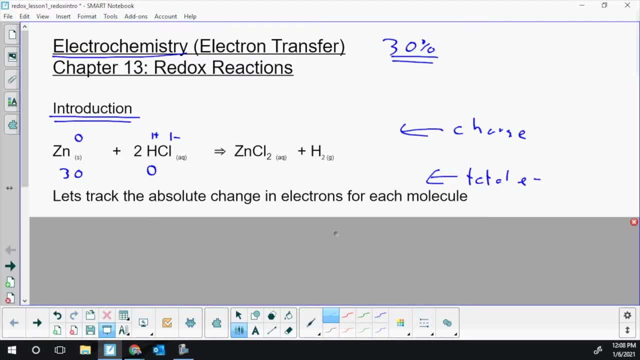 if we think, look at that chloride, that's Cl minus. chlorine is atomic number 17 and minus, it would have one extra electron instead of 18. now there is a two in front all of the charges and the electron counts that I'm writing is just for one one of the atom or the ion. so we've got a zinc with 30 electrons. we've 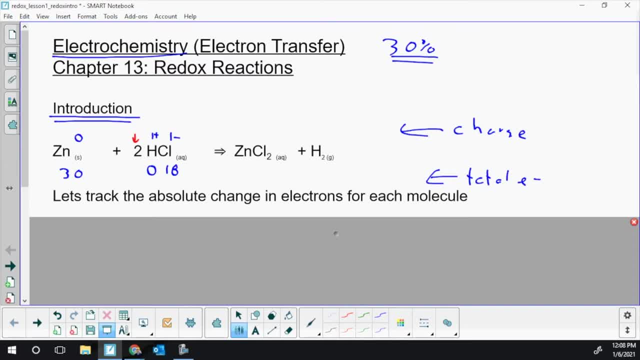 got an H. we happen to have two of them. they both have none and we have two Cl minuses and they're both 18. okay, now we're going to do the same thing for the other side when we get to the other side. I see zinc again, but it's no. 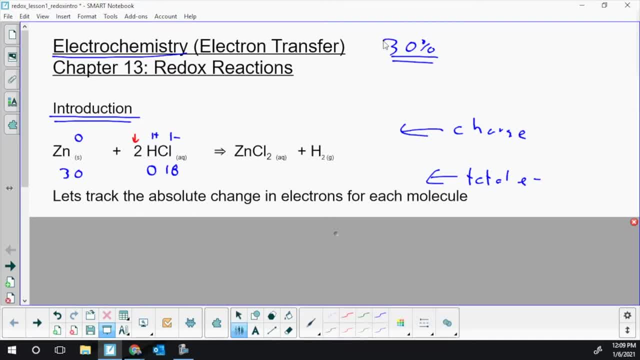 longer zinc neutral. we now have zinc in an ionic compound. that zinc is the two plus type. now one way you could get that charge is to is to look up chlorites charge and figure out what things would be. or if you Look in your data booklet. 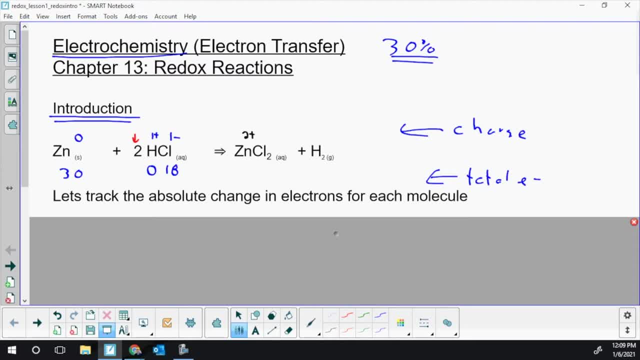 the only possible charge for zinc is is plus two, that's a two plus. please do a look and we'll see you then. So when I say your data booklet, I'm looking at just the inside of the front cover. It would be the very first page. 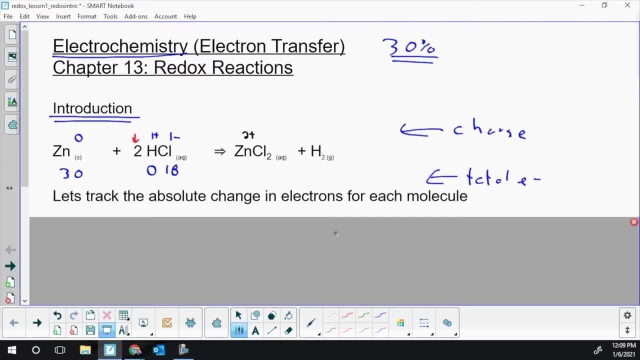 So that zinc is plus 2. So it no longer has 30 electrons, It's down to 28. That's the plus 2 type. Next we've got Cl. That's a Cl in an ionic compound. again, That's not diatomic chlorine. 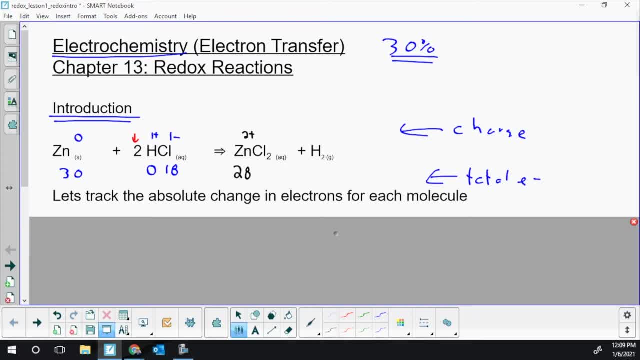 That's an ionic compound: one zinc, two chlorides. Well, that's exactly the same as before. We had a chloride back with a hydrogen in the beginning and we have a 1 minus Cl and each of those have 18 electrons. 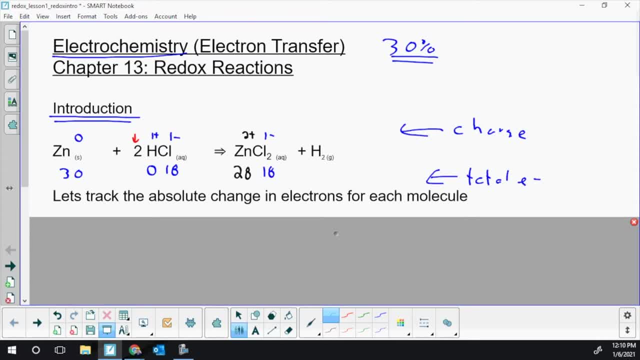 Again. I know there's two Cls. Each has 18.. It's not 18 in total. Last we have hydrogen. Now all molecules have no charge overall. Okay, In terms of electrons. I've been writing the electron count for each H. 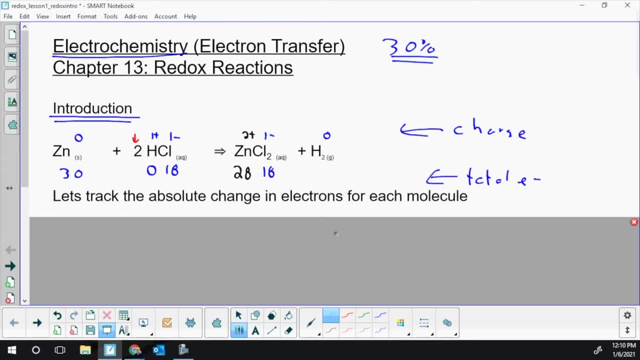 Here we've got two of them. So you know H2 looks like that Chem 20 bonding line. if I did an electron dot diagram That hydrogen has two. hydrogen molecule has two electrons. Now I've been writing the electron count for one. 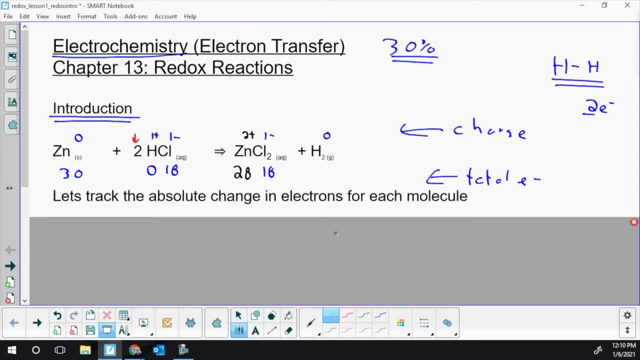 Of all of the atoms or ions. so I'm just going to. there's two electrons and there's two Hs. so I'm going to divide that by two. There's one electron for every H. So we start with zinc, with 30 electrons reacting with a hydrogen, with none. 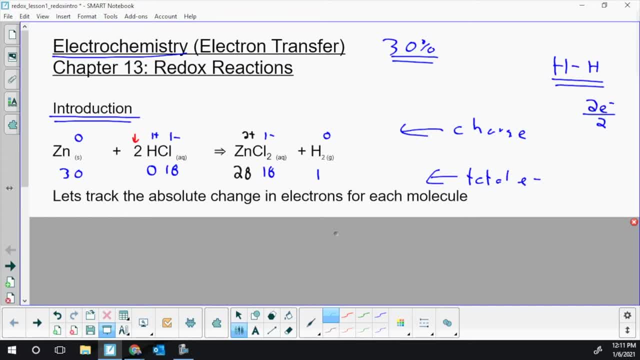 a chloride with 18,, making a zinc with a 28, a Cl with 18, and mixed diatomic hydrogen with one electron each. Okay, And now we can finally get at what's going on in terms of electrochemistry. So we're looking for changes. 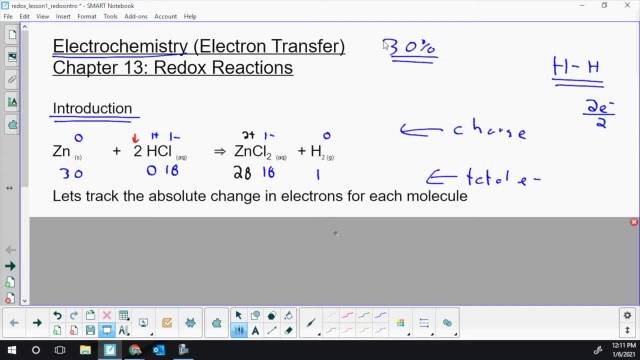 If I start with my zinc, that definitely changed. It went from 30 electrons at the beginning down to 28.. I did that arrow a little further than I wanted. There we go, zinc to zinc. We start with 30.. We end up with 28.. 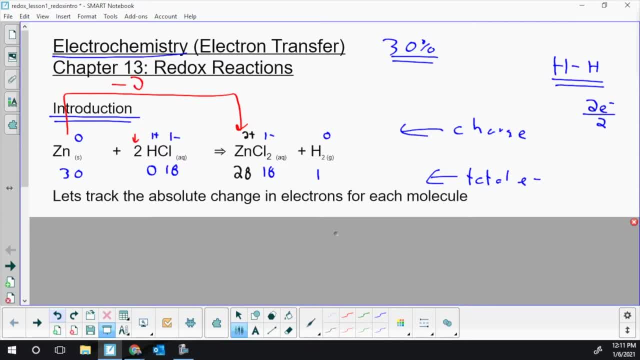 There is a loss, I want to go back. I'm going to go minus two electrons with that zinc to go from 30 down to 28.. Now in a reaction we're going to see that whenever you have a loss of electrons somewhere. 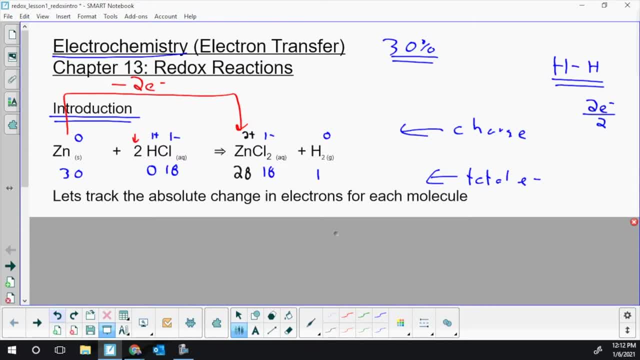 you have to have a gain of electrons somewhere else. So somewhere electrons were gained and that is with our hydrogen. Every hydrogen starts with zero and they end up with one on the product side, So there's a gain. so I'm going to write plus one electron with the hydrogen, okay. 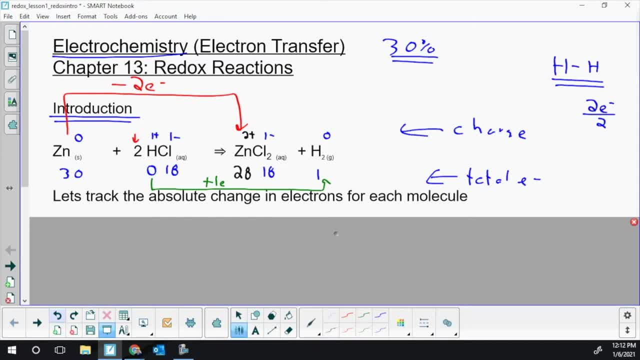 Now, just to be super clear, I'm going to put in or highlight minus one- sorry, minus two- electrons for every zinc. so I'm just going per zinc or slash zinc. With the green, it's plus one electron per every H. 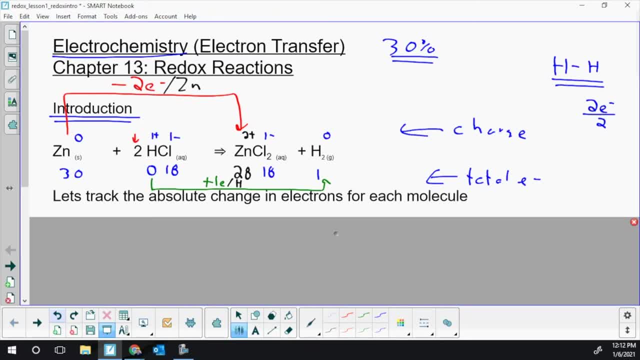 There's two H's, So in total there's a gain. So I'm going to write plus one electron with the hydrogen. In total there will be two electrons transferred, but it's one electron each. Now you can track electrons, like I did on the bottom, using the total count, but it's. 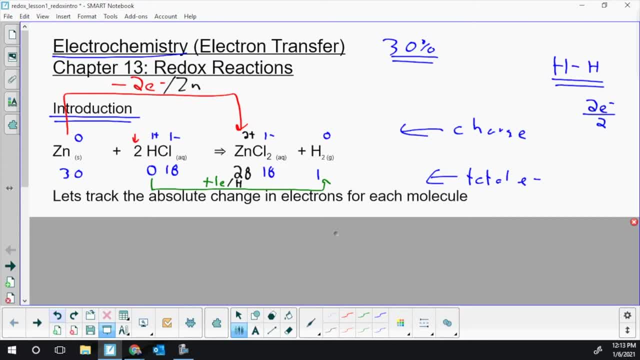 much faster and you get the same answer if you just look at the charge. So if you look at the hydrogen going from plus one to zero, okay, you get the same type of trend. So we've tracked the absolute change in each molecule. 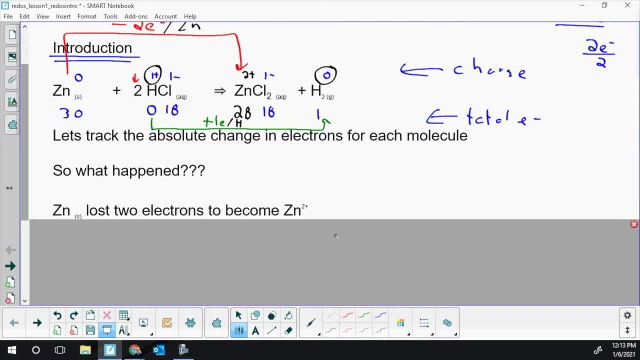 What has happened? Two big things have happened. Zinc lost two electrons to become zinc, two plus ion. That was the red. The other key piece is two H pluses gained, two electrons each to form molecular hydrogen. That's our gain and our loss, and we 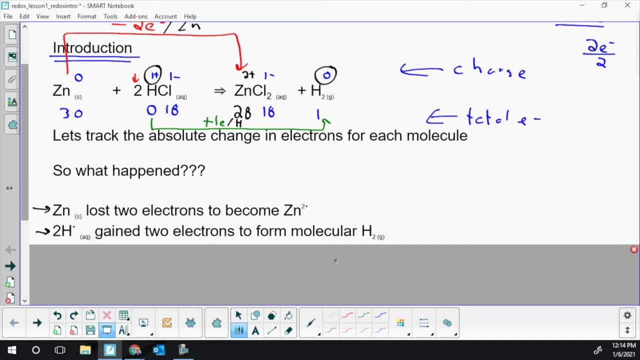 always have to have this pairing. Now there's one other atom that never showed up in the so what happened? statement, and that is Cl-. Cl- didn't do anything. It started with 18, it ended with 18, so it's just a spectator ion. 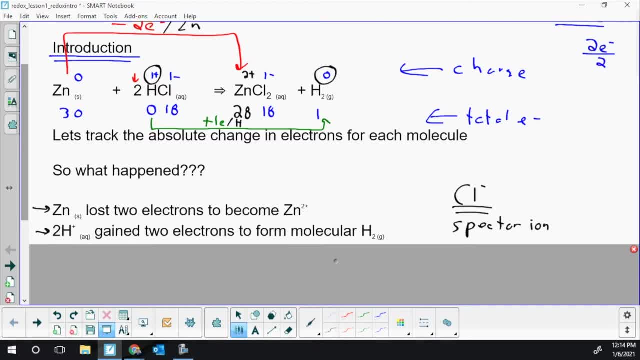 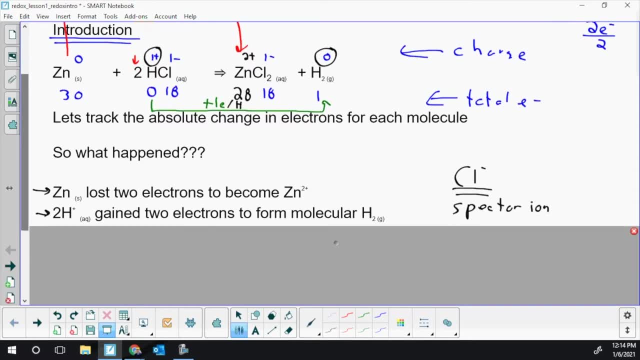 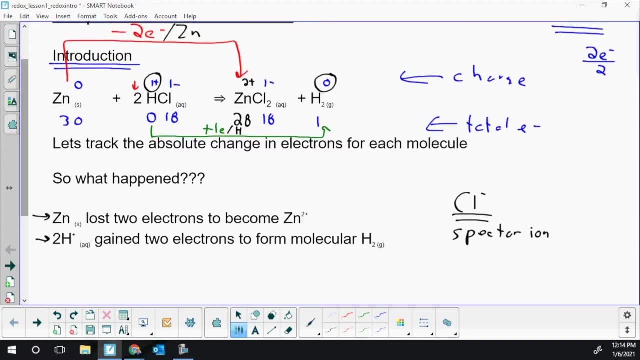 There is no electrochemistry, there's no gain or loss of electrons with our chloride. So the point of this slide was to find the two pieces, the gaining and losing of electrons, and now I want to talk about. well, there are distinctive names given to these names. First, key, fundamental definition. 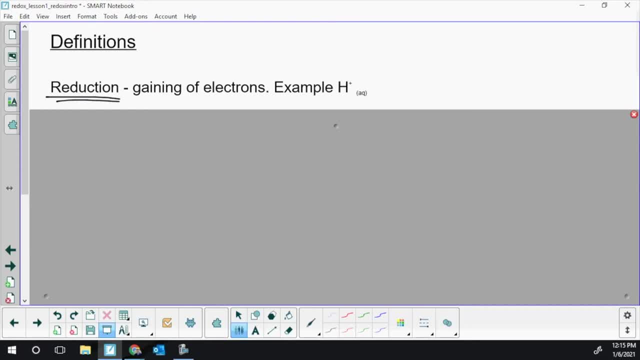 This unit is largely a terms, definition, understanding, type of unit. There is some math and calculations, but it's not a calculation heavy unit, It's more of a theory heavy unit. So reduction: That by definition is a process where there is a gaining of electrons. 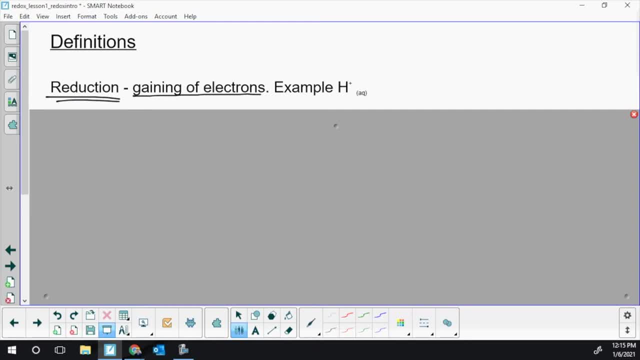 And in the example we just did, what gained electrons was the H+. When you gain electrons, your charge goes down because electrons are negative. The second key definition is oxidation, which is the loss of electrons, and the process that involves the loss of electrons. In our example, that was the. 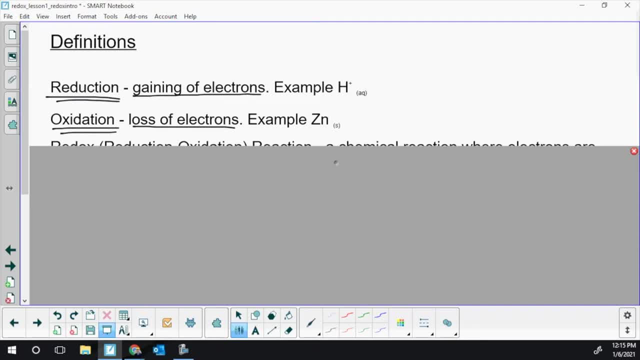 zinc metal. It started with 30 electrons and lost two. That's going to be the theme for the rest of this first lesson. When you put the two together- reduction and oxidation- you get a redox reaction, The reduction-oxidation reaction, The redox, the RE from. 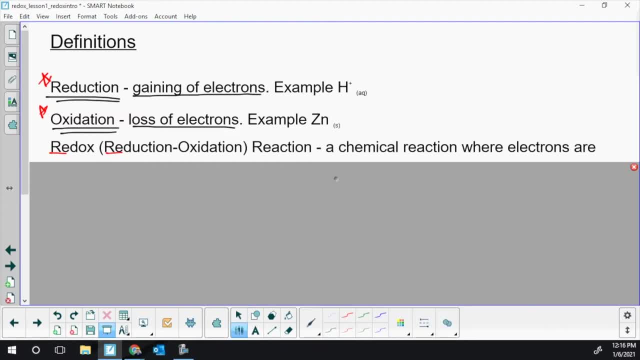 reduction. Sorry, the RED from reduction and the OX from oxidation. That's where the word Redox comes from. Okay, must have something losing and something gaining. not all chemical reactions are redox, and that's something we'll address in a future lesson. which type of 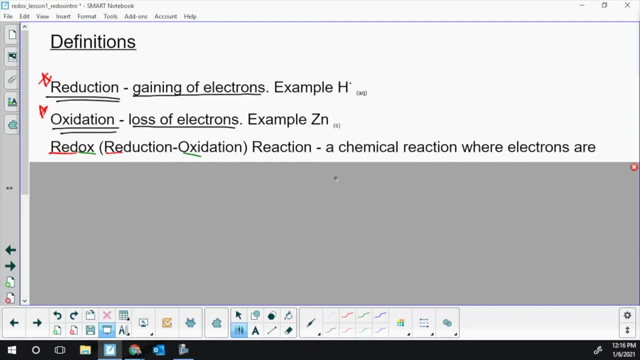 reactions are redox and which ones aren't? okay, we just saw a single replacement reaction and all single replacements are redox. so redox reaction, or chemical reactions where electrons are transferred from one of the reactants to another one of the reactants. in studying redox reactions, 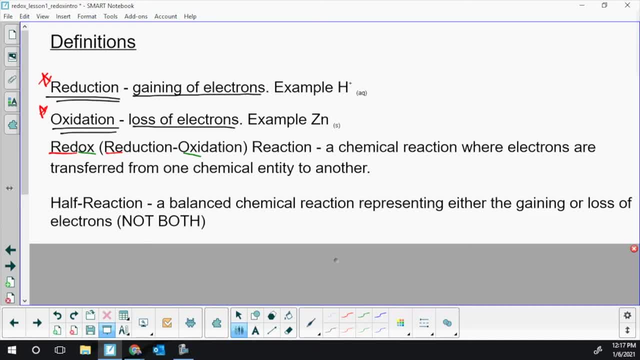 and this is how your data table on page seven is built- is by studying half reactions. they're a balanced chemical reaction that shows either the gaining or the loss of electrons. it doesn't show both. okay, the showing both would be a redox reaction showing just one of the two halves, one of the two pieces, the gaining or losing. 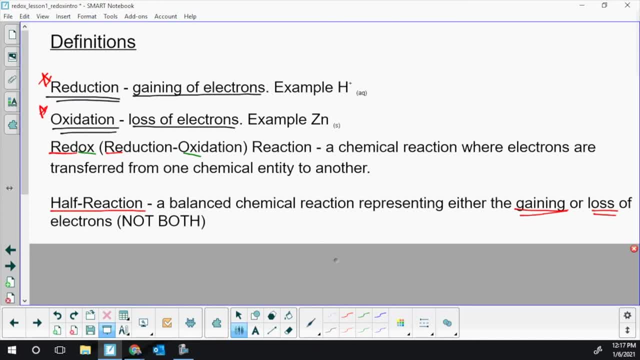 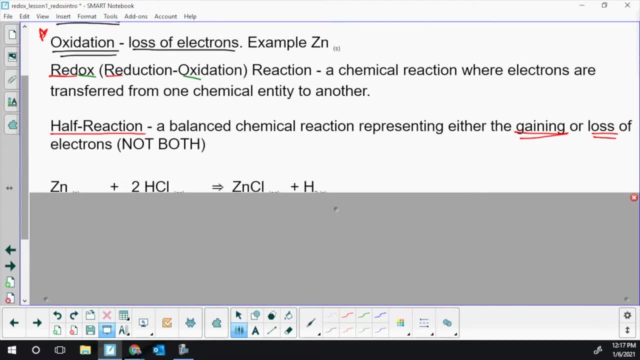 we call them half reactions. we're going to be writing lots of those and we're going to take a look at half reactions in the bottom of this slide. so I'm going to put back up that reaction that we looked at on the previous slide and we're going to write out the two pieces next. so I'm going to start with the. 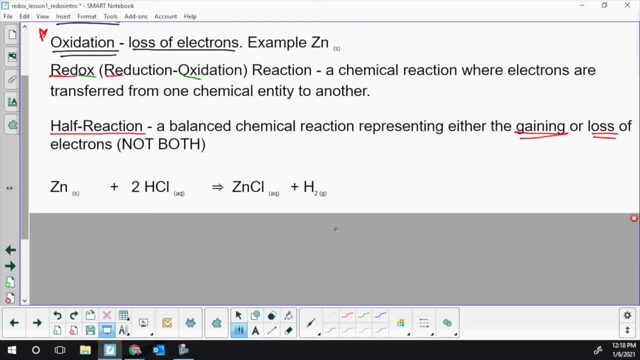 oxidation. so the oxidation area, our new definition is, that is, the loss of electrons or the process that lost them. So the loss was our zinc. Our zinc started with 30 electrons and ended up with 28.. So we only need to show those red underlined pieces in the oxidation. 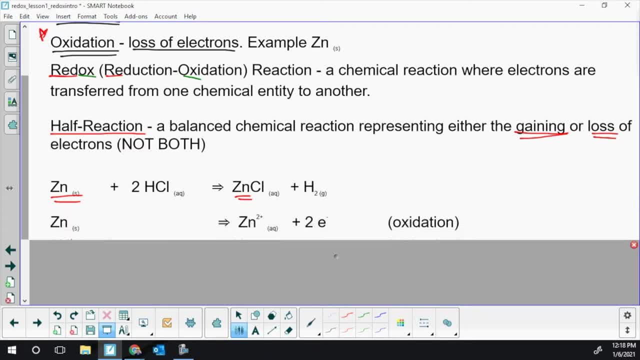 half-reaction. So I pulled down those red underlined pieces. So zinc solid is our only reactant in the oxidation half-reaction producing. the only product is zinc 2 plus. but then we've got to show the electrons that aren't shown in the single replacement, Zinc going from neutral down. sorry, 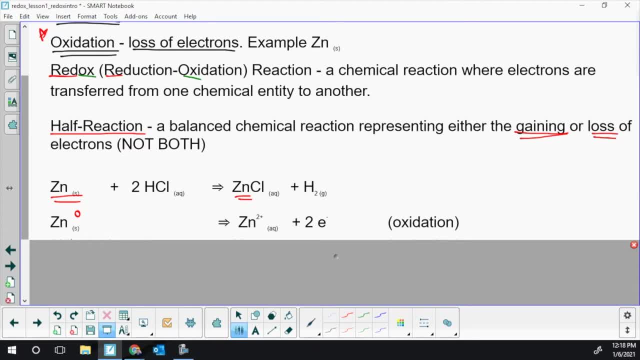 up to two plus involves losing two electrons. Any time electrons are lost, they're going to be a product. Any time there's a gain of electrons, they're going to be a reactant. So I'm writing: the oxidation electron are lost here, they're gonna have to show up on the product side, Our other half. 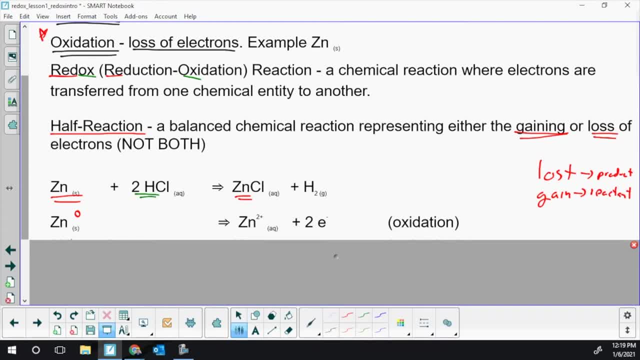 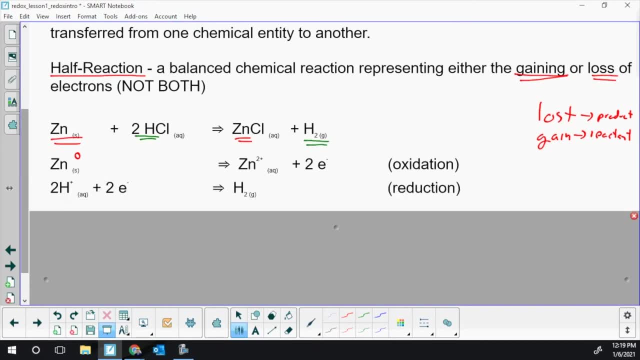 reactions involves our two H pluses producing elemental hydrogen. So that's what we see in the reduction half reaction. I've pulled down the two H pluses. It requires the gating of two electrons and we get our elemental hydrogen. And I'm not going. 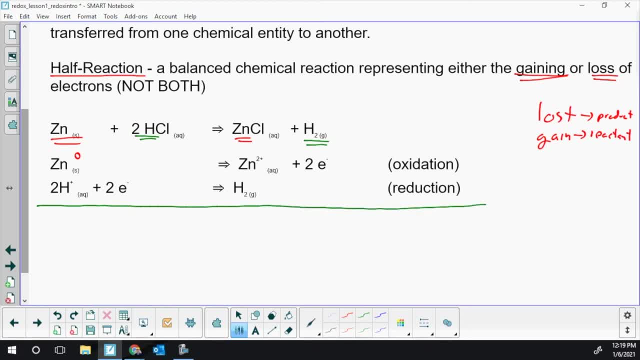 to write it out: If we netted these two reactions together, we would get the net redox reaction. Actually, I will write that out just so you can see it, When we write redox reactions, as you've been doing for years, of single replacement, 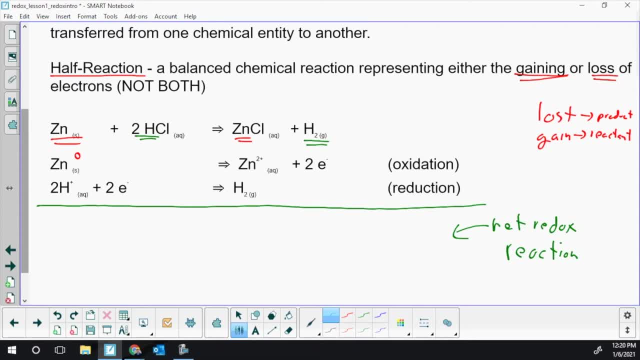 and not even realizing it. you never wrote the electrons in. They always cancelled each other out. We have two electrons from the oxidation and they're going to cancel out the two electrons from the reduction. So we don't see them in the net, We just see the zinc. 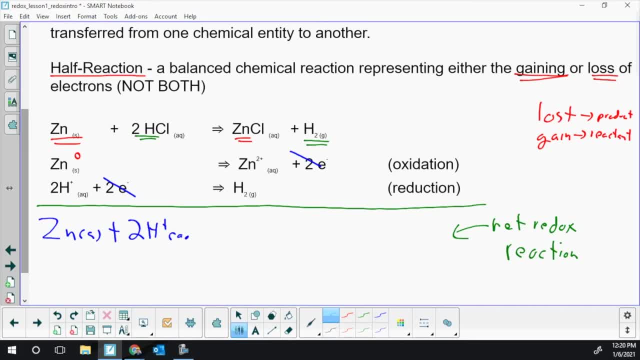 that loses electrons, the two H plus that gain them. We get the ionic zinc- The zinc after it's lost electrons, and we get the two H's molecularly bonded to each other when they've gained. Now you'll notice in the net reaction there is no chloride showing up. Spectator. 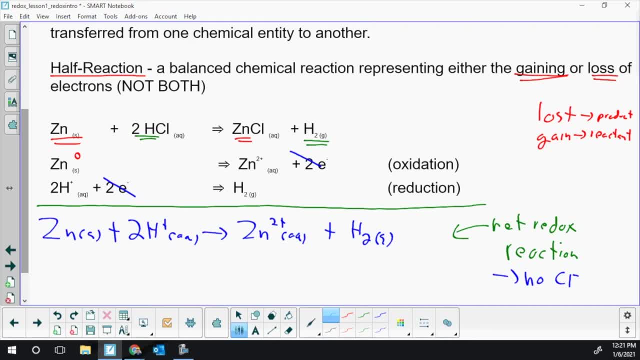 ions disappear when you put two half reactions together, Because spectator ions aren't going to show up in either half reaction. So we saw an example which led to our definitions of oxidation reduction. Next is a mnemonic: how are you going to remember this oxidation reduction? you just need to remember that. 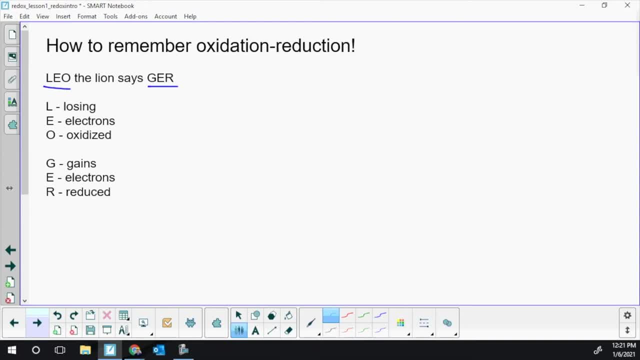 leo the lion says grr and you'll be fine. so leo helps me remember the oxidation part, grr. gaining electrons reduced, that helps me keep track. that reduction is the gaining part, oxidation is the losing. now, with lots of practice, you, you'll stop maybe saying leo and grr. 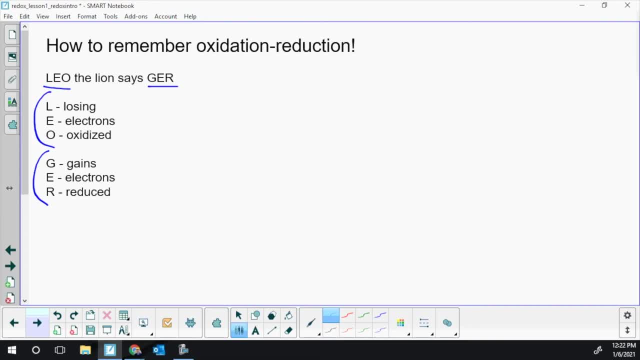 i'm going to write leo and grr all through my notes as a reminder for you. okay, it's not something you have to know, it's not something you have to memorize, it's just a mnemonic. so i'm going to do a couple more examples. give you some skills or tools. talk about your data. 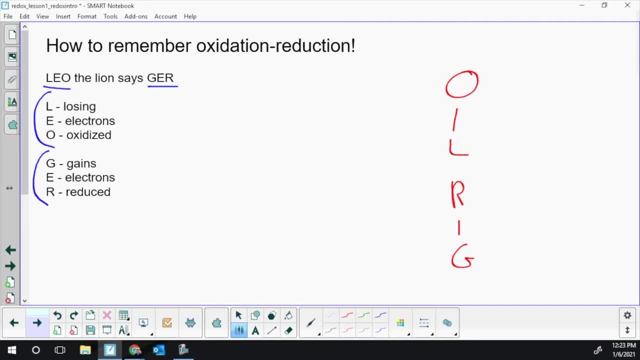 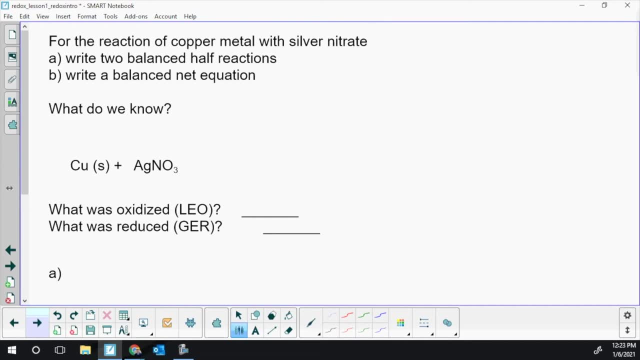 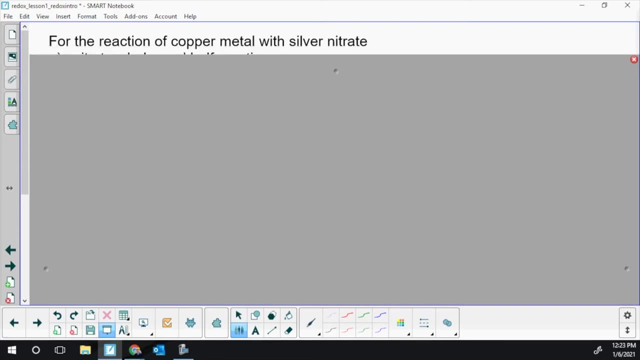 table and how that can help you. and then you're going to be ripping net reactions apart and figuring out what's the oxidation, what's the reduction, and you're going to do a couple more examples. so for the last example of this intro lesson, we're going to break apart, understand, uh, the 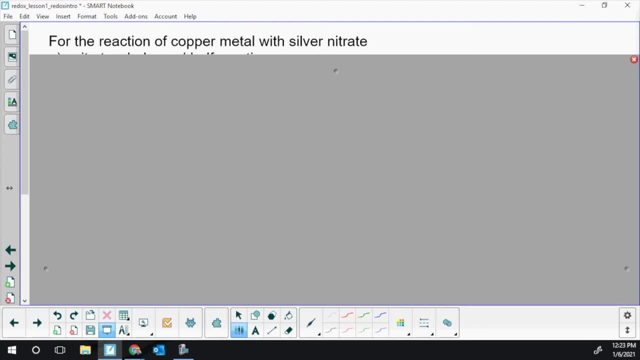 reaction of copper metal with silver nitrate, and i want to do a couple things. i want to write out two balanced half reactions, so an oxidation and a reduction, and i want to write out a balanced net equation. okay, now that net won't have any spectator ions in it. okay. 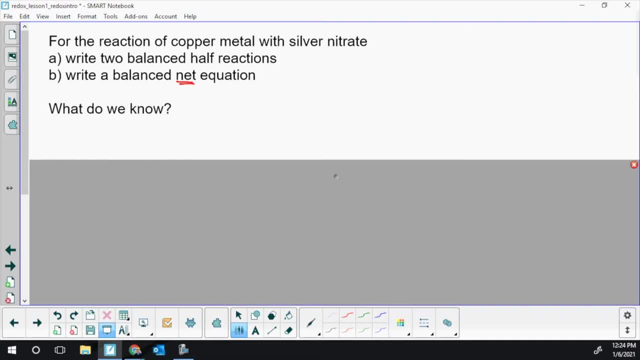 so i have to go back to my science 10 reaction type skills and think of which reaction type is this, because i didn't list the products for you. now we do have the reactants and words. copper metal- that's a metal by itself. all metals except for mercury are solid at room temperature, so that's where the solid came from. 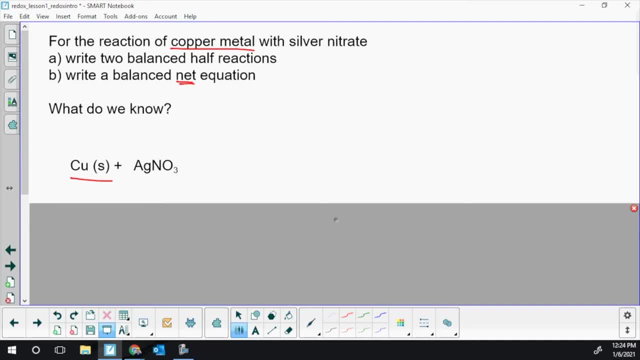 and killed by any amount of mercury. space does matter and metals by themselves are so, and metals by themselves are neutral. you don't have to write in the original charge. i'd actually would like you to write in the zero. so a lot of students like to always write charges in with metals, but when they're by themselves a 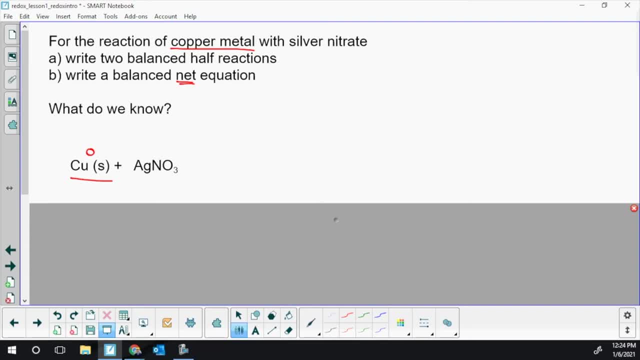 metal has no charge. the ionic compound that we think of as earth is also charged with a charge. so that you can estimate the charge, and in the same spin you might suggest that a charge would take all enjoy compound. it does have a charge. so that's our copper part. taken care of that. the second chemical is silver nitrate. silver in your 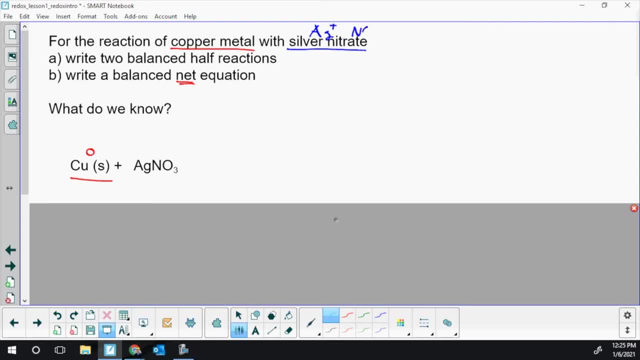 data table is positive. one nitrate is a polyatomic ion which is minus one, so we just need one of each of those. so that's why I wrote one silver and one nitrate, not putting the ones in now. I've got to predict the products before I can do any redox analysis. any thoughts, what type of reaction do I? 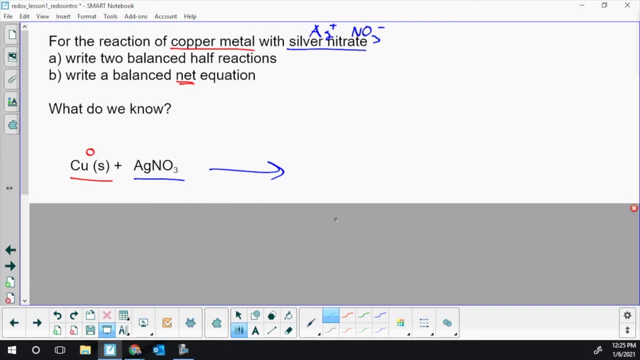 have here. I need to realize that in order to get products, so those five reaction types were combustion, single replacement, double replacement, decomposition and formation. and it is a single replacement, and so that's what I have to keep in mind. so in single replacement, the metals are going to 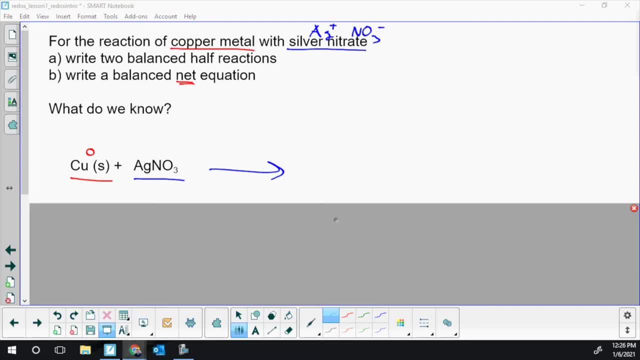 switch places and we have to, you know, think of their charges. so the copper is going to pair up with the nitrate now when it switches places with the silver, and then the silver is going to end up all by itself. now that copper isn't done, I have to figure out what charge that copper is and that 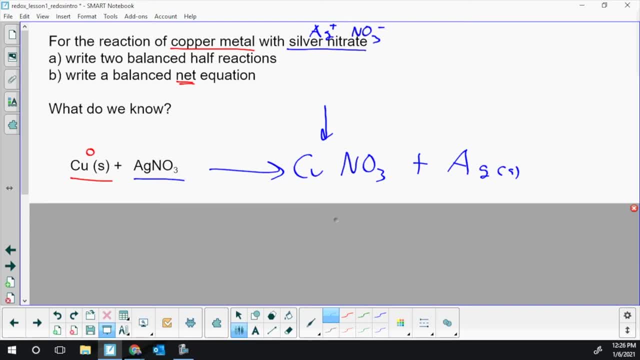 tells me how many nitrates I need. so this is where I need to go to my data table right inside the first cover and look up what is the most common charge for copper. hopefully somebody has their data booklet. what is the most common charge for copper? and it is plus-two. it is two types. 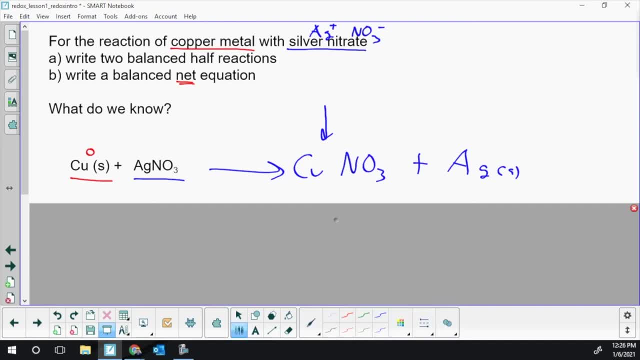 but the plus two is written first. so this is plus two copper, copper. this is one minus nitrate. so to make this balance, I need two of those. so now I've got the products out, I just need a balance, this whole thing, and then I can start trying to figure out what's going on. redox wise, I got one copper at 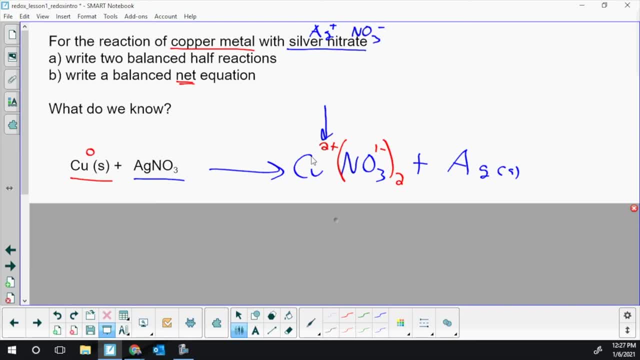 the beginning, one copper at the end, one silver at the beginning, one silver at the end, one nitrate at the beginning, two nitrates at the end. so to fix my nitrate I have to put a two in front of my silver nitrate. that doubled my silver. 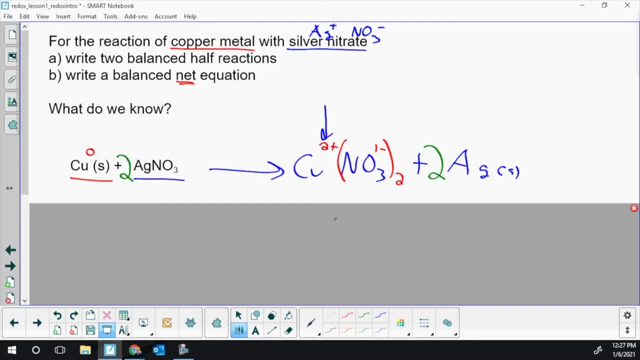 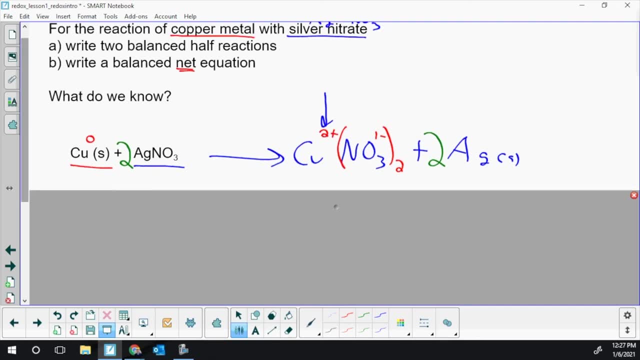 I double my silver at the end. and now I've got my balanced equation. so now I'm going to start diving into part a. let's start trying to figure out what would oxidize and what was reduced. so what was oxidized- and our mnemonic, remember that is losing electrons- is. 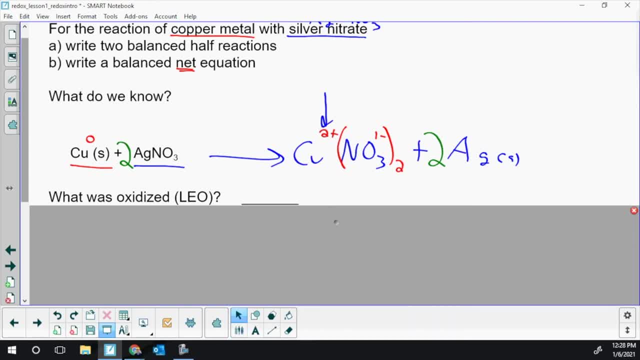 oxidized. I want to throw in some charges. that is silver one plus we got nitrate, a polyatomic ion. I won't dive into all those pieces yet and I'll just label this is neutral silver as our product. okay then, no three doesn't change at all. 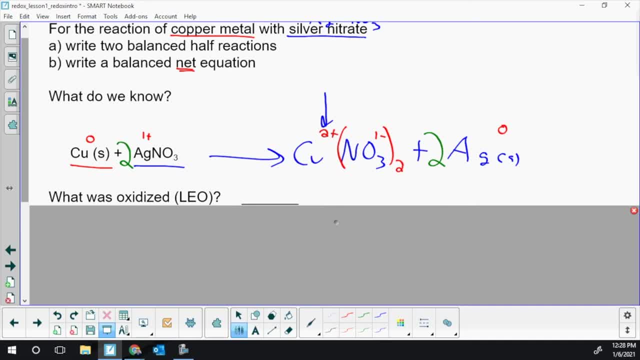 and when we see something not changing the charge or the count of atoms in an ion, there's going to be no electrochemistry there if we look out. so what lost electrons? copper started with zero and ends up plus two. zero to plus two, that would be losing electrons. you have to lose two electrons. 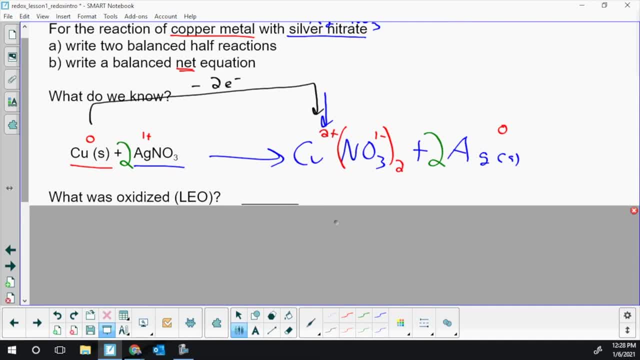 to end up positive. so what was oxidized? that is our solid copper reactant. thanks, we're gonna have to write a half reaction with just the copper. what was reduced? so that's our grr. what gained electrons? that's going to be our silver. it goes from plus 1 and it goes down to zero. 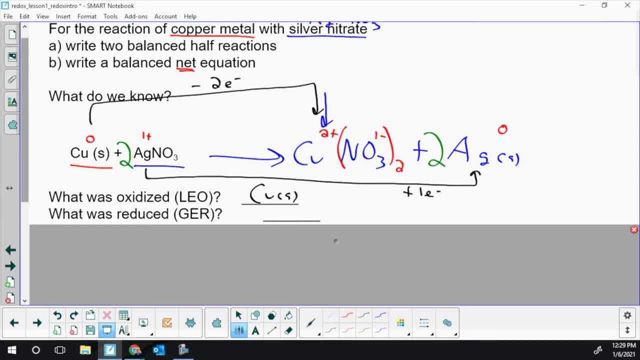 it gains one electron. now get all. these numbers are two electrons per copper and one electron per silver. okay, so what was reduced? which reactant was it? it's the silver plus. okay, I'm not going to include the nitrate, it's just the silver that gained electrons. so now, 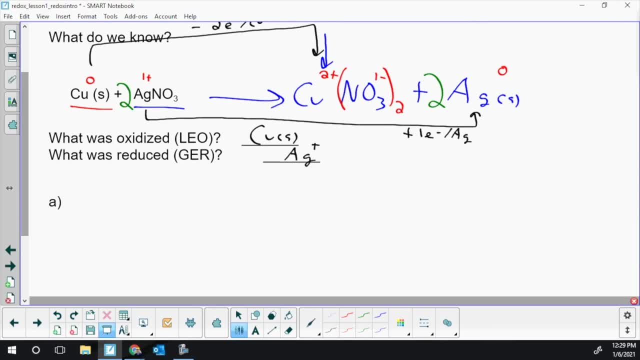 I can write a couple half reactions, knowing what was oxidized and what was reduced. so I'll start with the Leo. so the oxidation, which always has the electrons as a product. we had solid copper becoming copper 2 plus and there's a difference of two electrons. 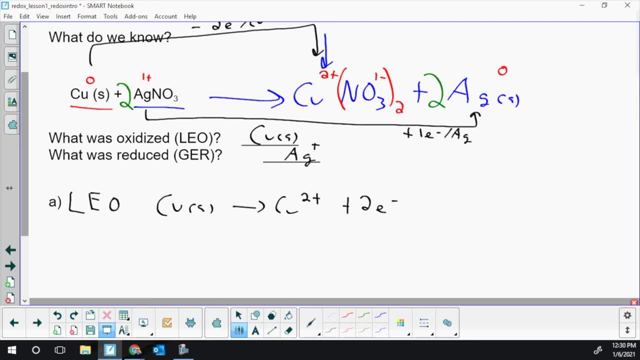 there our reduction, our grr gaining electrons reduced. so this better have electrons at the beginning. we have silver and that's silver plus and that picks up one electron, it gains one, and then we get neutral silver. you don't have to put the zero charge in, but I really encourage you to put those in. so 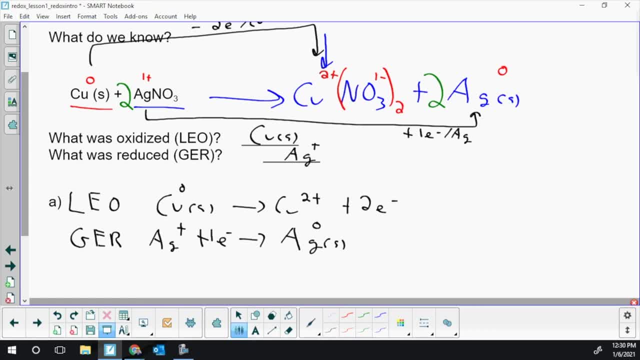 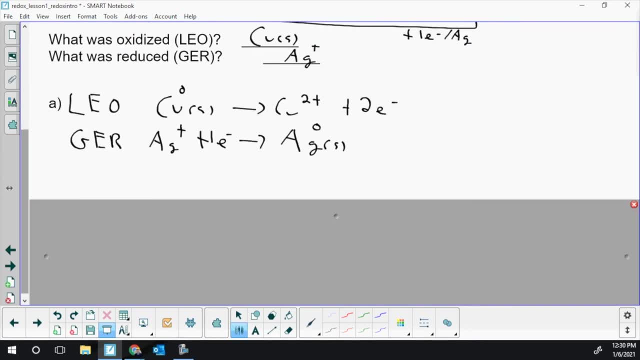 that's part a done. we figured out the oxidation. we figured out the gaining. last B: what is the net? well, to get a net redox reaction, you have to put two half reactions together. so we're going to add the two half reactions, but we do have to balance the. 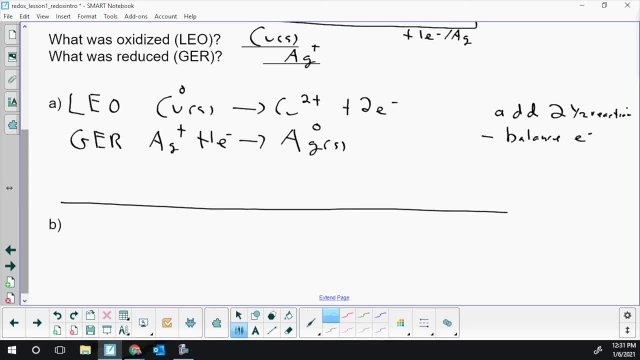 electrons before we do it. when we look at these two half reaction, I've got two electrons in the first half reaction and I only have won. and second, when we write half reactions they're always written with the lowest possible coefficients but I hope the half reactions on page 7 are constructed in that. tell you when. 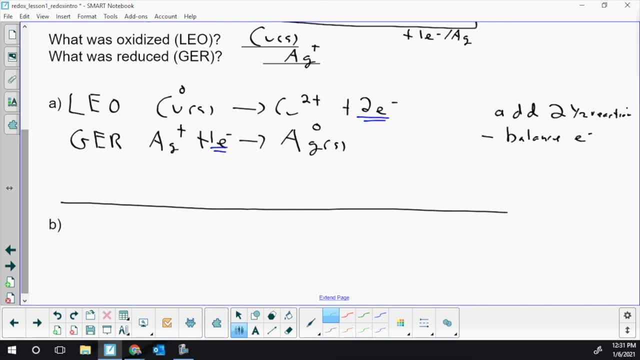 we're going to construct them when we not reactions up. we often have to multiply one or both reactions to find the lowest common multiple of electrons. in this case, the lowest common multiple between two from the copper and one from the silver is two electrons. I have two. 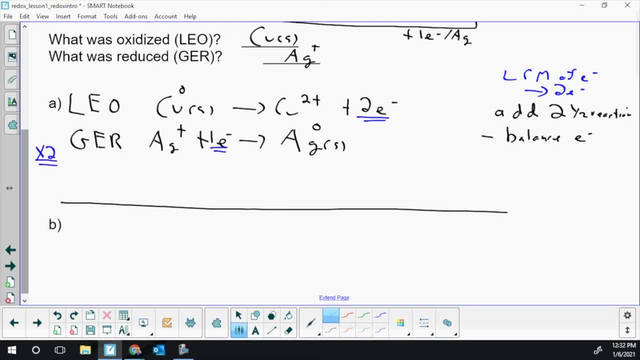 electrons in the top, I have to double the bottom reaction to get two. so I need two silver plus and two electrons producing two neutral silver. okay, the half reaction is the black. the blue that I put over top of it is manipulating it to build the net and that leads to me being able to cancel my 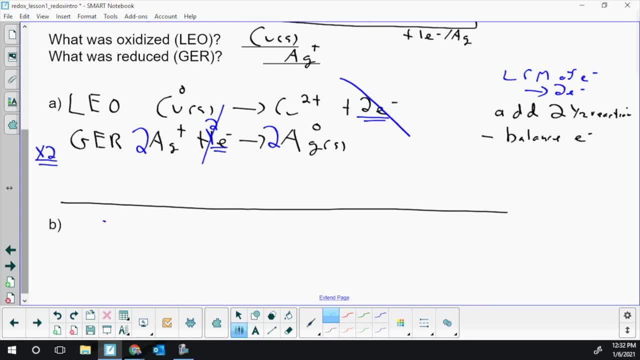 electrons to build my net and I end up with copper solid plus two silver plus producing copper two plus and neutral solid plus producing copper two plus and neutral solid plus two silver plus producing copper two plus and neutral solid plus producing copper two plus and neutral silver. and our spectator, ion of. 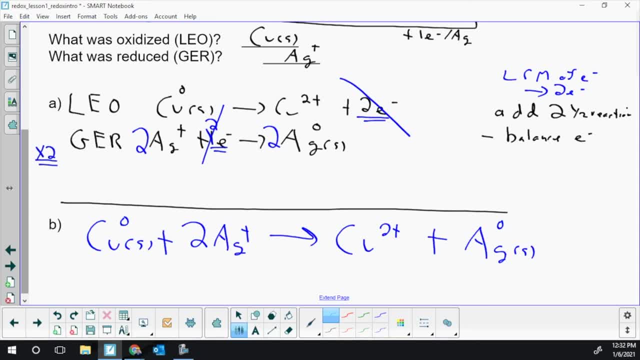 silver two plus and neutral silver and our spectator ion of silver two plus and neutral silver and our spectator ion of nitrate disappeared because it's not silver and our spectator ion of nitrate disappeared because it's not silver and our spectator ion of nitrate disappeared because it's not involved in any electron exchange. what nitrate disappeared because it's not involved in any electron exchange. what nitrate disappeared because it's not involved in any electron exchange, what we're seeing here is the heart of involved in any electron exchange. what we're seeing here is the heart of involved in any electron exchange. what we're seeing here is the heart of batteries, and that's what we'll look at. 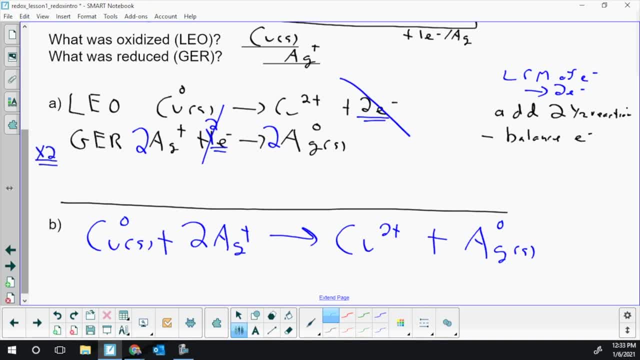 we're seeing here is the heart of batteries and that's what we'll look at. we're seeing here is the heart of batteries and that's what we'll look at in chapter 14. if you separate these batteries- and that's what we'll look at in chapter 14- if you separate these two chemicals and make the electrons not go, in chapter 14. if you separate these two chemicals and make the electrons not go in chapter 14. if you separate these two chemicals and make the electrons not go from chemical to chemical and solution. two chemicals and make the electrons not go from chemical to chemical and solution. 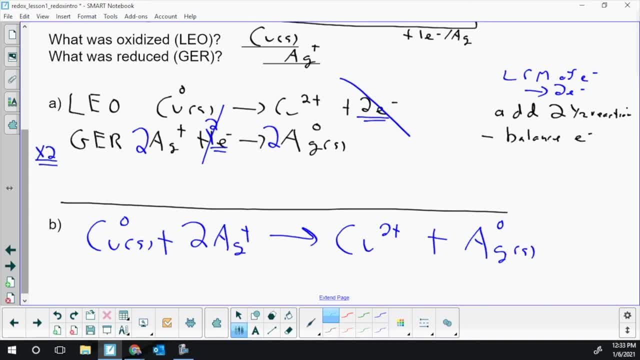 two chemicals and make the electrons not go from chemical to chemical and solution but run through a wire. you can power your from chemical to chemical and solution but run through a wire. you can power your from chemical to chemical and solution but run through a wire. you can power your iPhone. you can power, you know, any electrical. but run through a wire. you can power your iPhone. you can power, you know any electrical, but run through a wire. you can power your iPhone. you can power, you know, any electrical device you want and in today's world you can iPhone. you can power, you know any electrical device you want and in today's world you can. 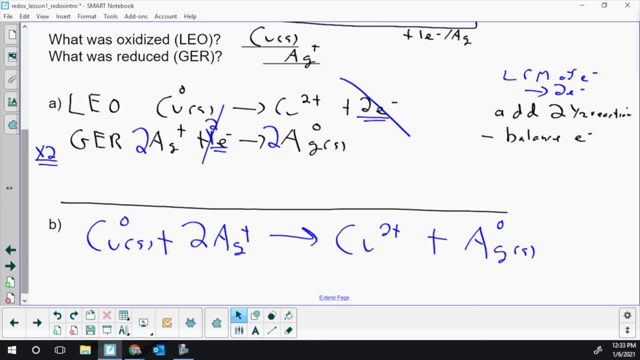 iPhone, you can power, you know, any electrical device you want and in today's world you can power an electric vehicle with the electron power, an electric vehicle with the electron power, an electric vehicle with the electron flow. so a few skills tools for you. flow. so a few skills tools for you. 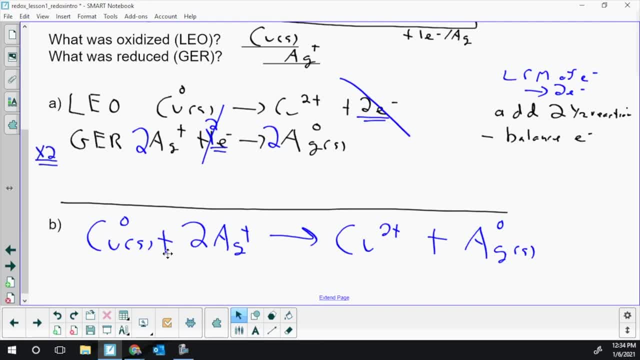 flow. so a few skills tools for you, and then you're going to be practicing in a, and then you're going to be practicing in a, and then you're going to be practicing in a couple minutes. so the first big tool I: couple minutes. so the first big tool I 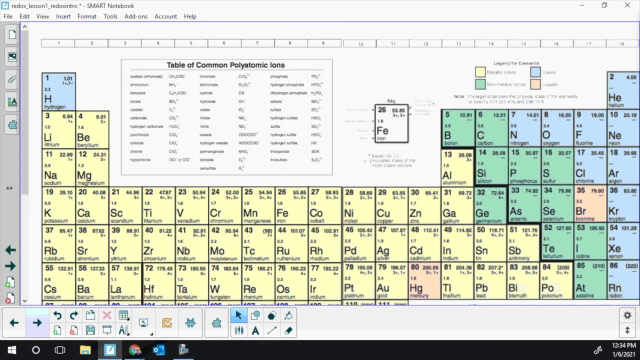 couple minutes. so the first big tool I was using and talking about is this data was using and talking about. is this data was using and talking about? is this data tape? is your data table? okay, you're tape. is your data table? okay, you're tape. is your data table? okay, you're going to be flipping through this all the 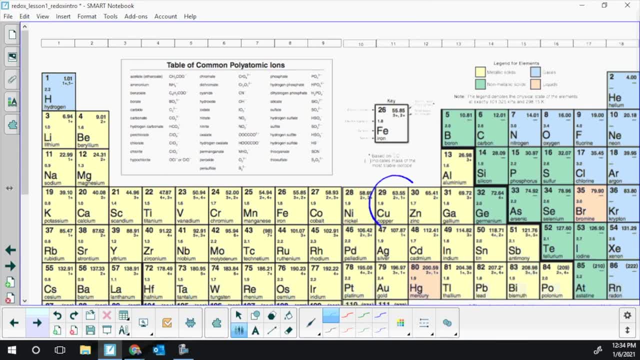 going to be flipping through this all the going to be flipping through this all the time in single replacement reactions. time in single replacement reactions. time in single replacement reactions- like we just saw you'd have to be. like we just saw you'd have to be. like we just saw you'd have to be looking for copper to find out what is. 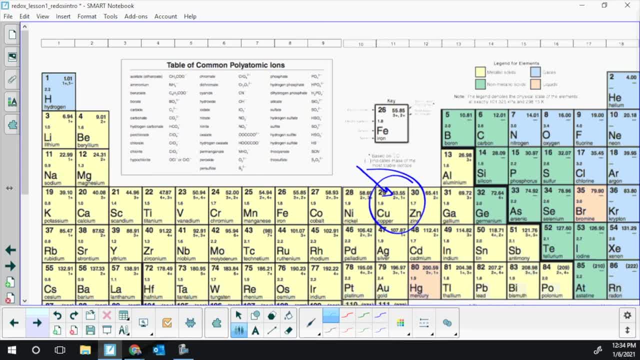 looking for copper to find out what is looking for copper. to find out what is the most common charge now your group. the most common charge, now your group. the most common charge now your group. one and two metals are a bit simpler all. one and two metals are a bit simpler, all. 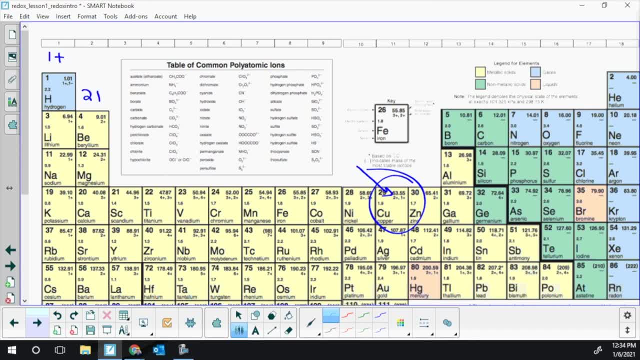 one and two metals are a bit simpler. all the group ones are one plus and all the the group ones are one plus and all the the group ones are one plus and all the group two metals are two plus. when group two metals are two plus, when group two metals are two plus when they're ionic, when they're by themselves. 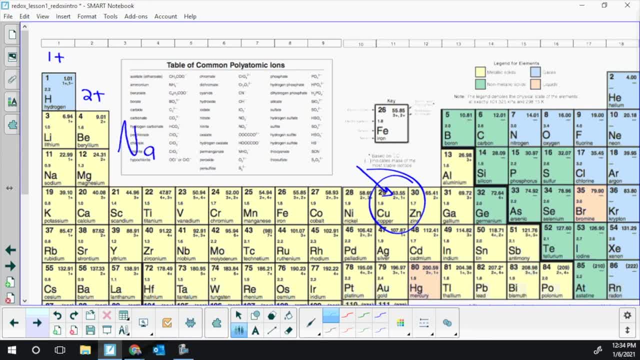 they're ionic when they're by themselves. they're ionic when they're by themselves. they are neutral. if you have sodium, all they are neutral. if you have sodium, all they are neutral. if you have sodium all by itself, it's not plus one, it's neutral. 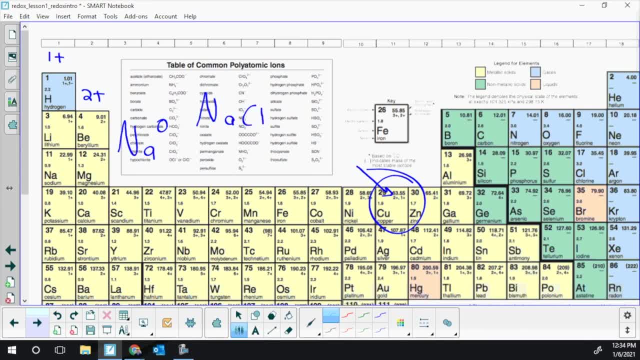 by itself. it's not plus one. it's neutral by itself. it's not plus one. it's neutral. it's only when you have sodium with it's, only when you have sodium with it's, only when you have sodium with something else that you have it as a. 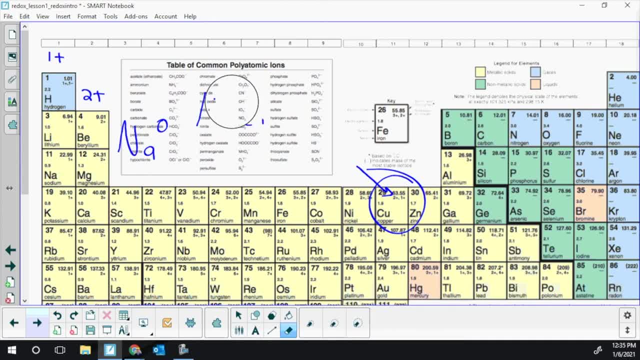 something else that you have it as a something else that you have it as a charge species. okay, so to get charges charge species. okay, so to get charges charge species. okay, so to get charges that aren't listed in questions. you're that aren't listed in questions, you're. 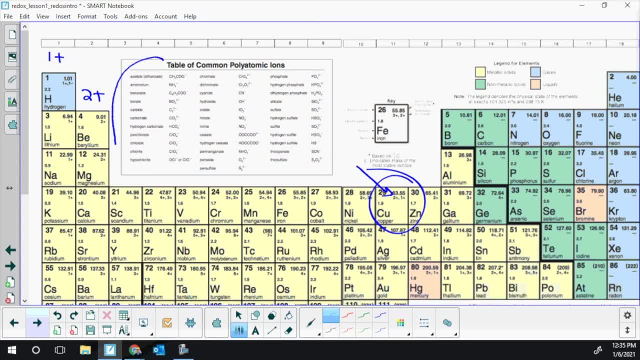 that aren't listed in questions. you're expected to go to your table. you're expected to go to your table. you're expected to go to your table. you're going to see lots of polyatomics again. going to see lots of polyatomics again. going to see lots of polyatomics again, like nitrate that we just saw and those. 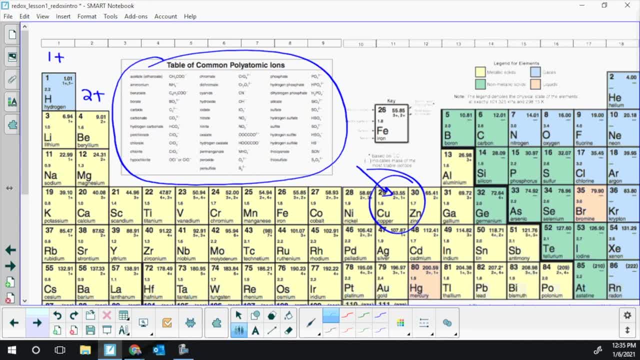 like nitrate that we just saw and those like nitrate that we just saw, and those names are all in that table. so that's names are all in that table. so that's names are all in that table. so that's the first tool. that's really useful. 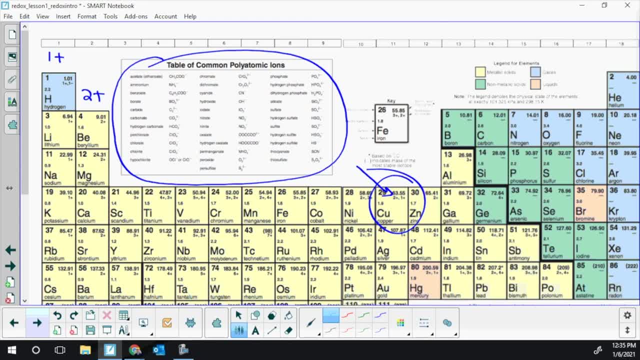 the first tool that's really useful. the first tool that's really useful, essential for you to be looking up those. essential for you to be looking up those, essential for you to be looking up those charges. the second key tool, this is charges. the second key tool, this is: 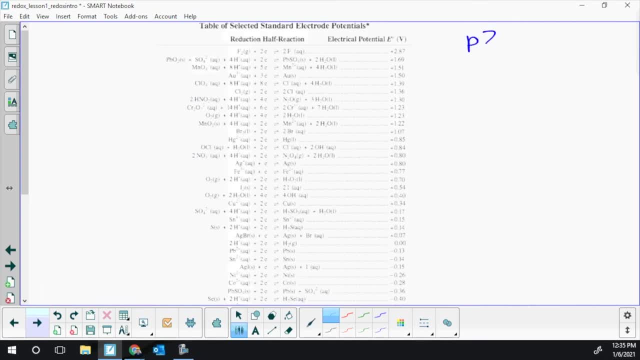 charges the second key tool. this is really blurry, but this is your data really blurry. but this is your data really blurry, but this is your data table from page seven. this is a table table from page seven. this is a table table from page seven. this is a table filled with reduction half reactions. 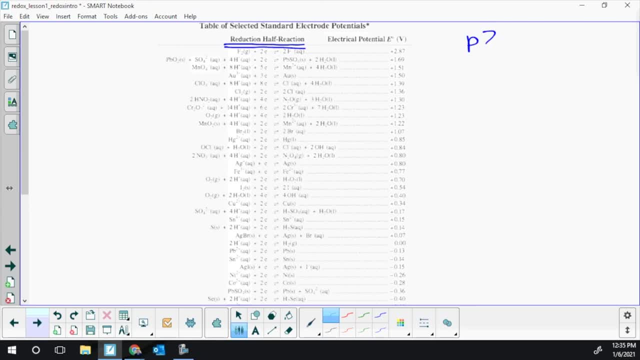 filled with reduction half reactions. filled with reduction half reactions. and you're always going to have this table and you're always going to have this table and you're always going to have this table. on tests and exams: okay so when? on tests and exams: okay so when. 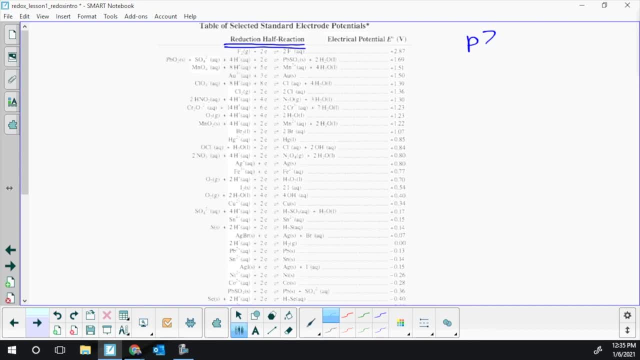 on tests and exams. okay, so, when you're back when we're doing our first quiz, or you're back when we're doing our first quiz, or you're back when we're doing our first quiz or a unit test at the end, this is a unit test at the end. this is. 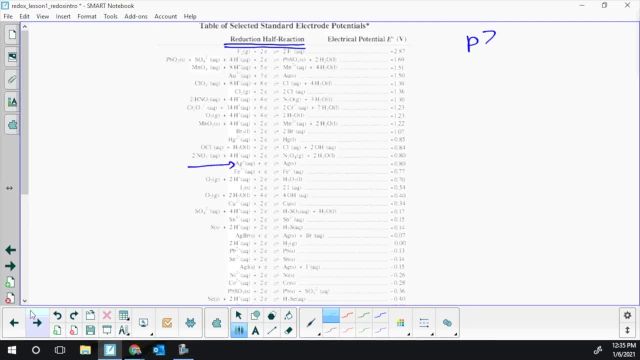 a unit test at the end. this is there for you and you'll see if you look in there for you. and you'll see if you look in there for you and you'll see if you look in your table, that whole silver half, your table, that whole silver half. 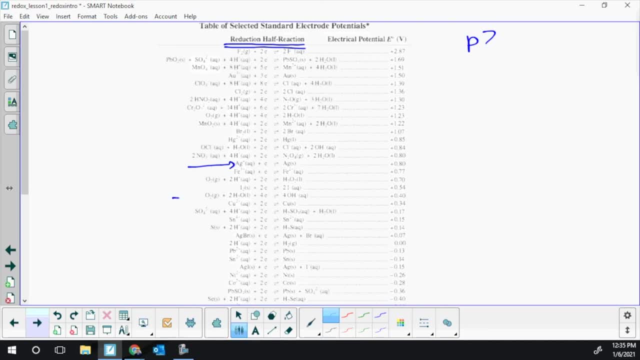 your table. that whole silver half reaction is right there in your table. reaction is right there in your table. reaction is right there in your table. and that copper half reaction we're just and that copper half reaction we're just. and that copper half reaction we're just looking at is in the table. but your 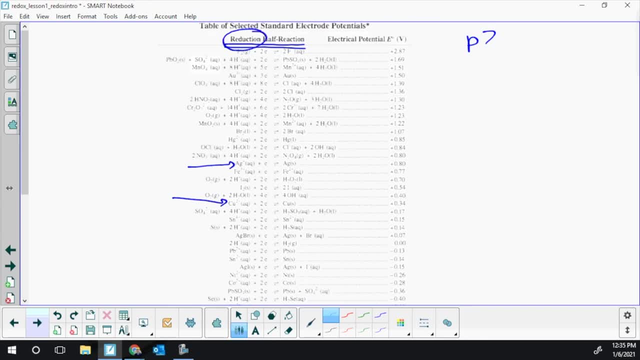 looking at is in the table. but your looking at is in the table. but your table has them all written as reductions. table has them all written as reductions. table has them all written as reductions. okay, your table is built as a ger table. okay, your table is built as a ger table. 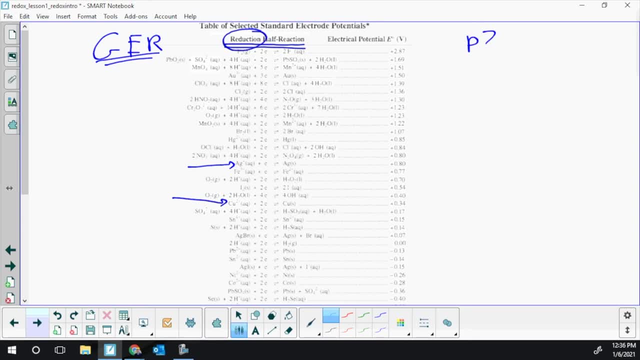 okay, your table is built as a ger table, a gaining table where all the electrons. a gaining table where all the electrons, a gaining table where all the electrons are on the reactant side. okay, and we'll are on the reactant side. okay, and we'll are on the reactant side. okay, and we'll talk even more about this table in. 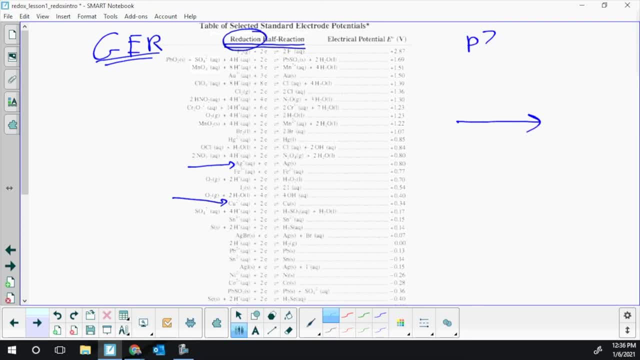 talk even more about this table in talk even more about this table in lesson two. the last thing, I'll just lesson two, the last thing, I'll just lesson two. the last thing I'll just highlight if you think of the forward, highlight if you think of the forward. 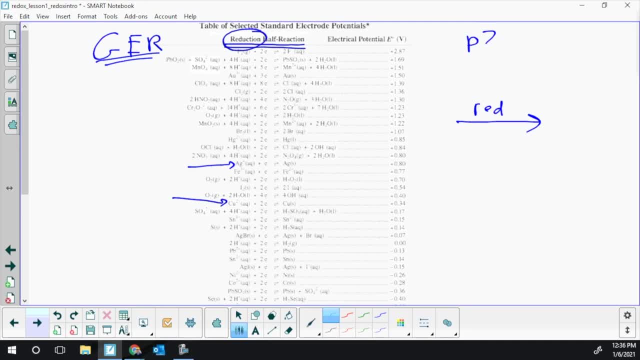 highlight. if you think of the forward direction of this table, it is a direction of this table. it is a direction of this table. it is a reduction. if you go backwards, so if you reduction, if you go backwards, so, if you reduction. if you go backwards, so if you think of starting with copper and going, 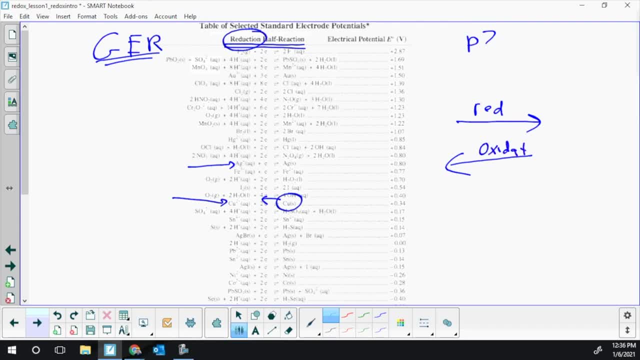 think of starting with copper and going. think of starting with copper and going backwards. that is an oxidation. so it's a backwards. that is an oxidation. so it's a backwards, that is an oxidation. so it's a reduction table, but you can get. reduction table, but you can get. 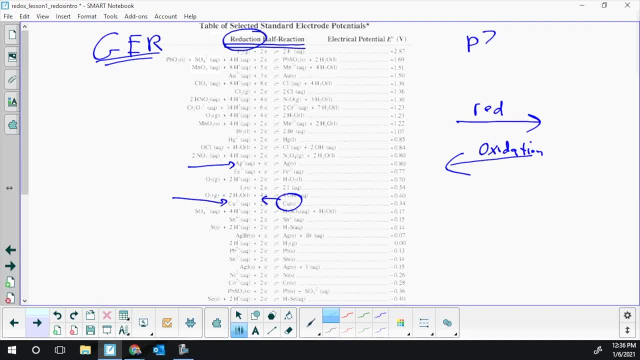 reduction table. but you can get oxidations by working backwards. oxidations by working backwards. 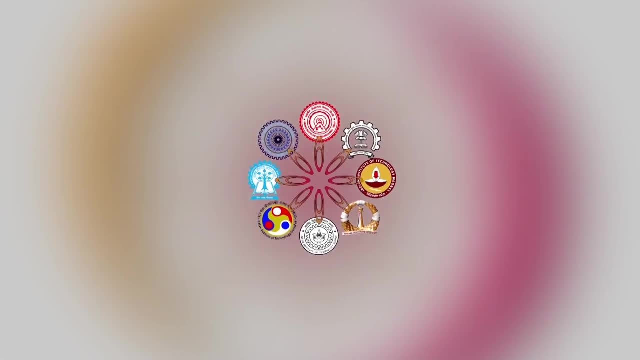 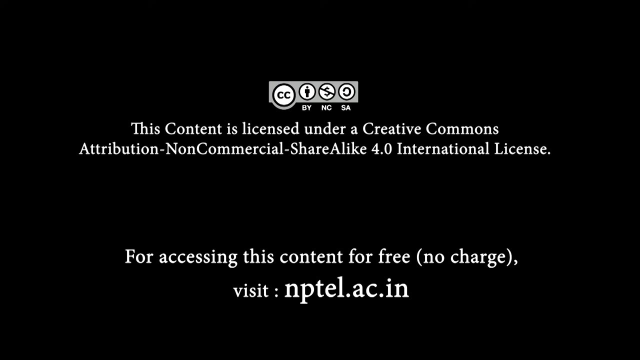 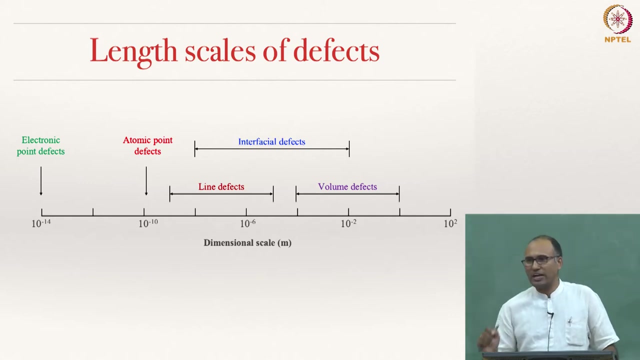 So we have looked at point defects and then we also said what are the different kinds of defects that we have discussed in the last class? Subatomic defects, like where you need to have an electron and if the electron is not there in the material, then it becomes.